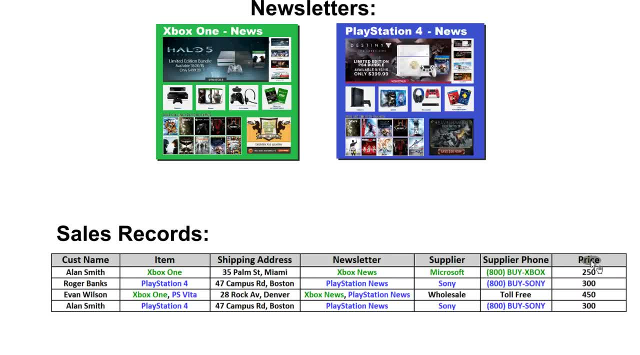 what is the phone number of the supplier and what is the price of the purchase. So they have someone named Ellen Smith. These are just imaginary Items, But anyway there's somebody named Ellen Smith. He bought an Xbox One. He lives in Miami, He subscribed for the Xbox newsletter. The supplier for the 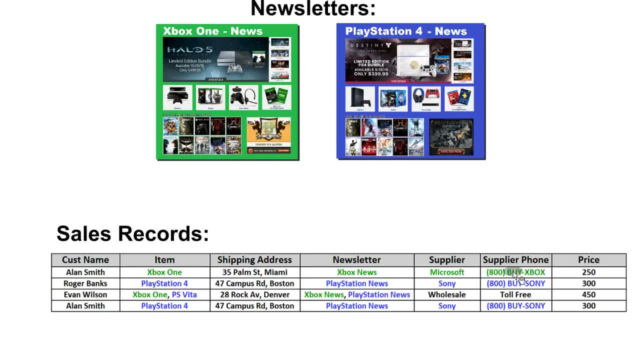 Xbox is Microsoft and their phone number is 1-800-BUY-XBOX, And the price was $250.. The next person named Roger Banks. he bought a Playstation 4.. He lives on campus road in Boston. He subscribed for the PlayStation. 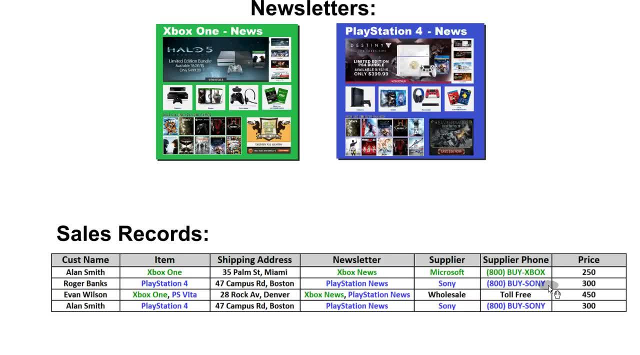 news and that was supplied by sony. their phone is by sony and the price of that was 300.. the next person, evan wilson. he bought xbox one and a playstation vita. he lives in denver. he subscribed to both newsletters and the supplier. it says wholesale and the supplier phone number. 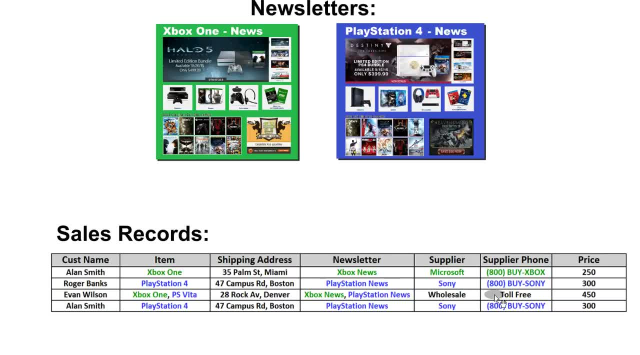 is stall free. this is what somebody entered in here, and the total price was 450.. and there's another item, uh, named ellen smith. it's the same as this, at least the name is the same. this person bought a playstation 4.. he also lives on campus road in boston, which is the same address as for. 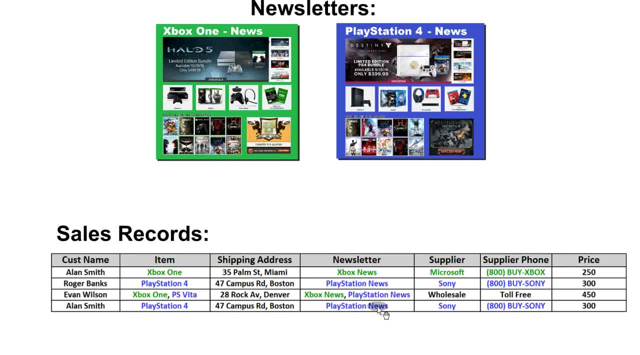 this person, roger banks. he subscribed for playstation news sony, buy sony and the price was 300.. uh, and the color code? just ignore the color code. there's no meaning to that, it's just for visual cue. so anyway, these are some of their sales records and i'm going to normalize these. so 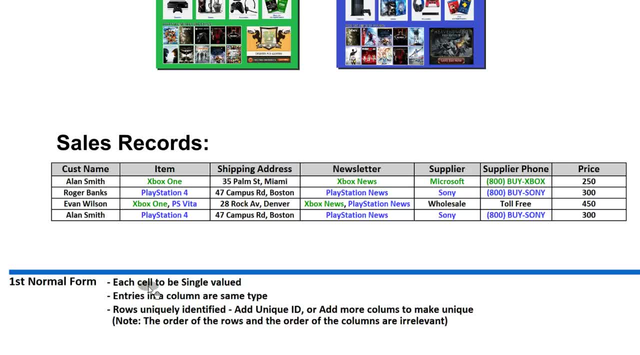 first normal form. the criteria is that each cell to be single value. so xbox one and playstation vita occur in the same cell. so is this? so we have to eliminate that. uh, entries in the column are the same type, so this one says wholesale and toll free here. these are not the same. these are not the 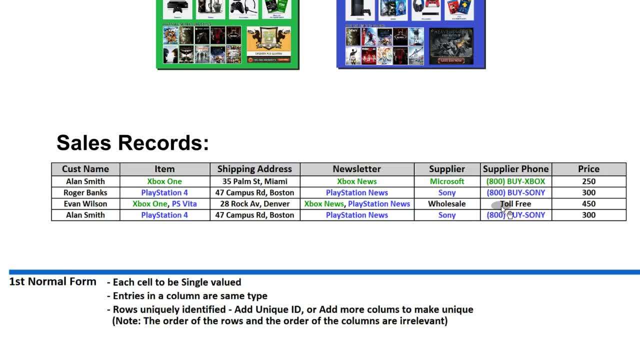 same type of values. so we need some kind of uh entry here that matches these. it would be like if, let's say, this field would be eye color and someone put like, uh, i don't know blue or green and beautiful. well, beautiful is not a color, it's an opinion. so we need some kind of uh actual. 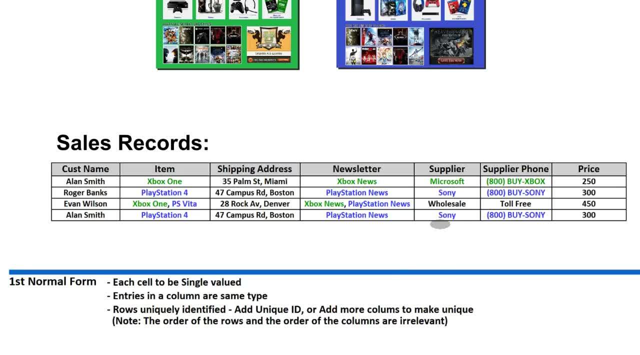 entry. we can't, we can't let this be in here. uh, also rows uniquely identified. so with the rows here, you can either add a unique id or add more columns to make the rows unique. well, these rows: there's no duplicates in these rows, so they unique in a way, but there's still. 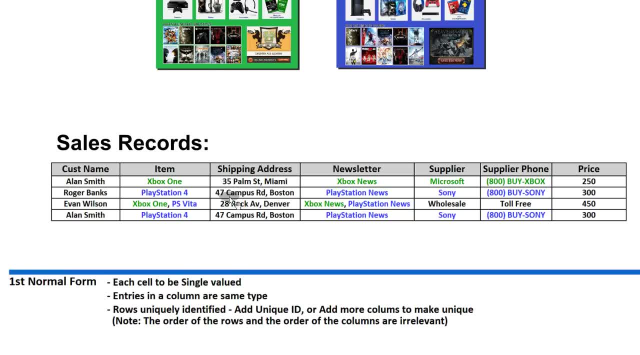 a question about this, ellen smith. well, this campus road in boston happens to be a housing for a college, so this this roger banks. he's in college and Alan Smith also rents the same house with them. they rent it together, so they have the same address while they are in college. so the 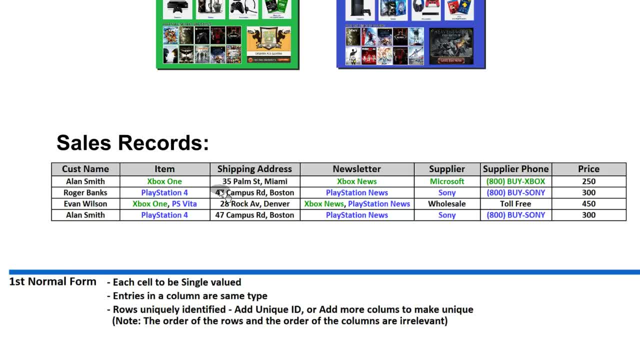 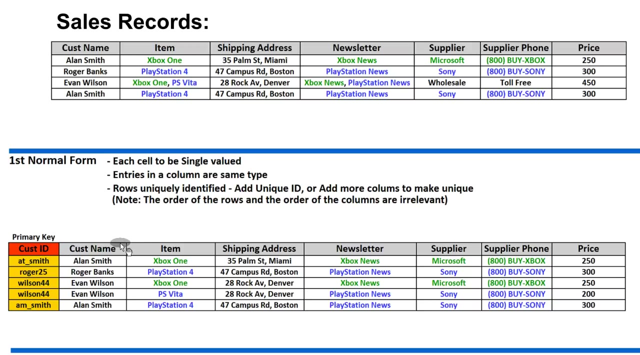 question is now: is this: Alan Smith, from Miami, is going to college in Boston and this is the same guy is just now, this is his address, or they are completely different people from this table. we cannot figure that out. so those are the issues. so this is the table in first normal form, so each cell to be single. 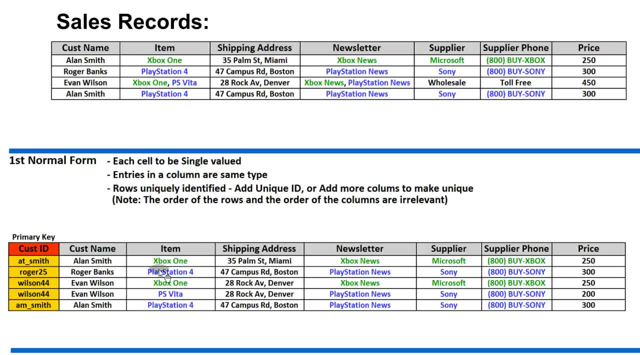 valued. so the Evan Wilson, these two items was separated out to two separate rows, one for Xbox one and one for PlayStation Vita. notice this has four rows here and then the button here this has now five because he made two purchases in one transaction. so that takes care of that entry in the column. are the same type? well, wholesale and. 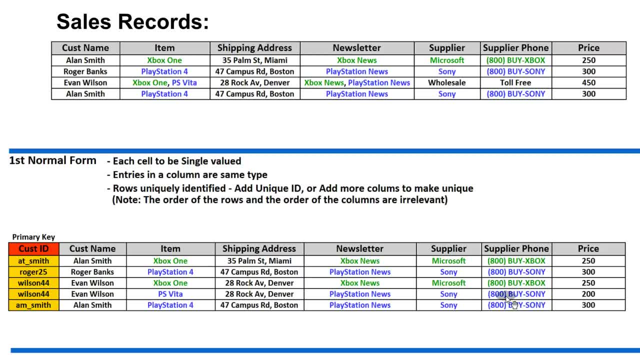 toll-free was replaced with the proper values. so now we don't allow entry of just random values in here. they have to be filled out properly and the rows must be uniquely identified. so these people are made to create some kind of customer ID that they can sign up, sign in to this website. so this person, his name, happens. 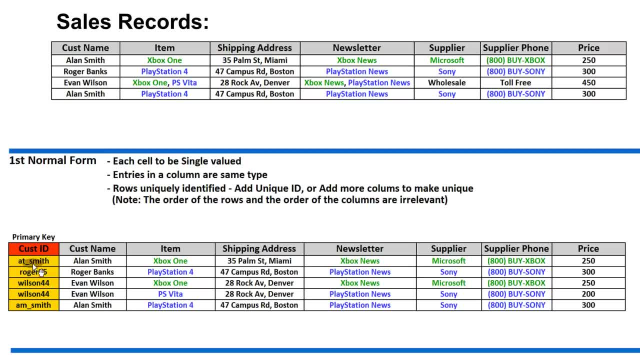 to be Ellen Thomas Smith, so he created a user ID: 80 Smith. Rogers Bank has Roger 25. Evan Wilson is Wilson, 44, and this person he had his name happens to be Ellen Michael Smith, so he is. his user ID is am Smith. so now we know for sure that these two people have. 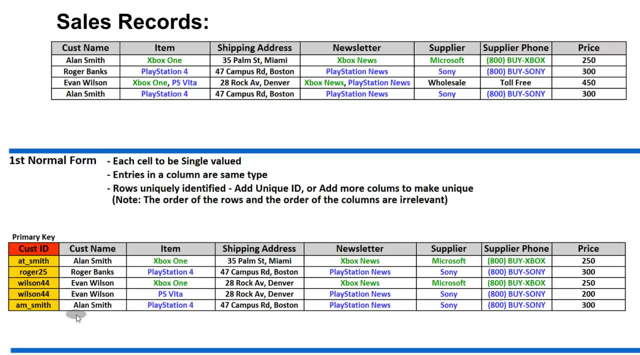 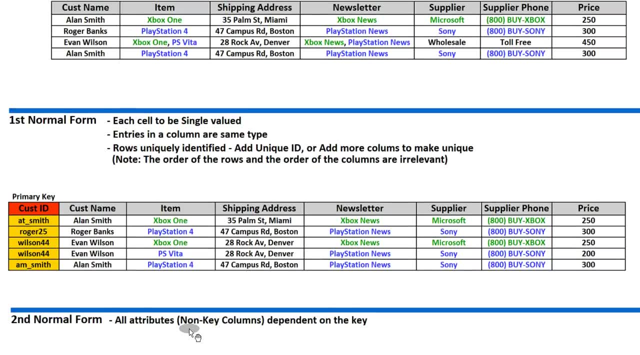 nothing to do with each other, and now we can uniquely identify each of these customers. ok, second, normal form: all attributes, meaning non key columns, meaning these, these white ones, dependent on the key. which is this one, this red? so which one of these don't depend on the key? well, 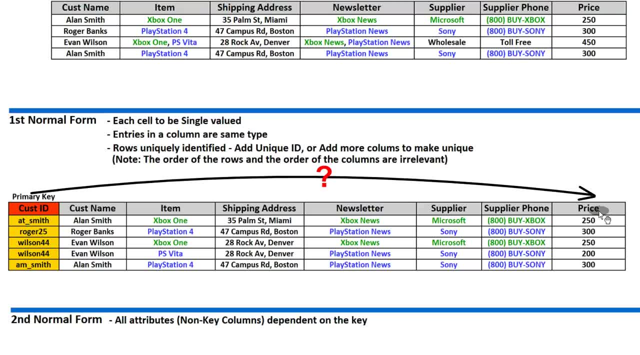 let's see how. about the price? so does the customer ID determine the price? in other words, does the price depend on who buys it? and the answer is no, doesn't matter who buys an Xbox one. the price will be the same when, when Alan Smith or Evan Wilson buying, the price will be the same. so 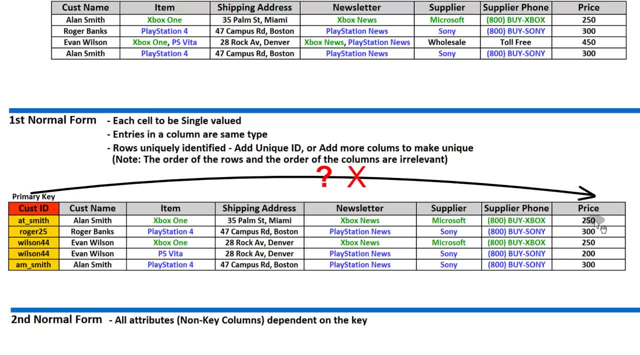 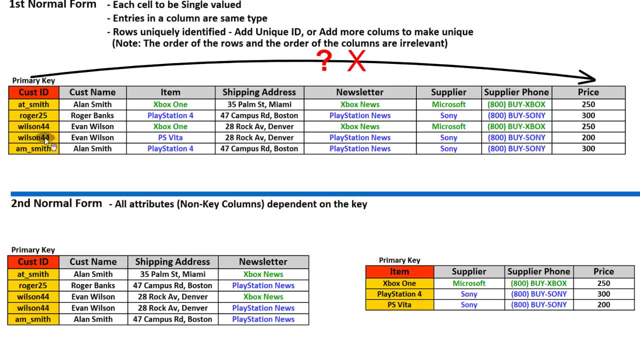 the. the key in the table doesn't determine this, so that we have attributes, meaning columns, that don't depend on the key. so those have to be separated out. so what I did is I take the customer ID, the name, shipping address and the subscription into one table. 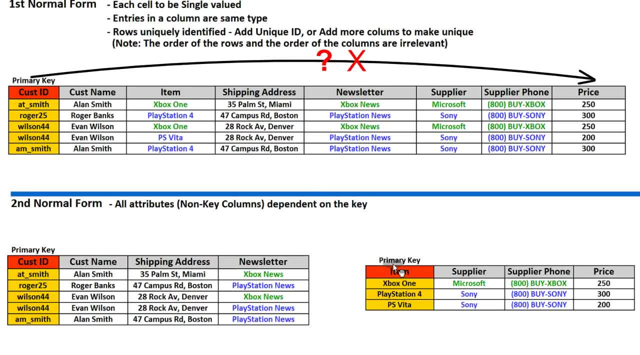 then I take the item which becomes the primary key in the other table- the supplier, supplier phone number and the price- into another table and obviously I'm only gonna list one item one time. so now the price, the supplier and the supplier phone and the supplier depend on this because Xbox one has Microsoft. 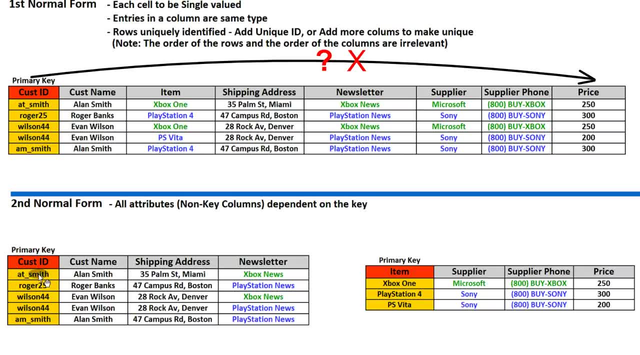 supply. this is their phone number and this is the price and this customer has. this is his name, this shipping address and this is what is subscribed to. obviously, this person subscribes it too, so he's in here twice. so this is great. the only problem is we lost the transactions. we don't know who bought. 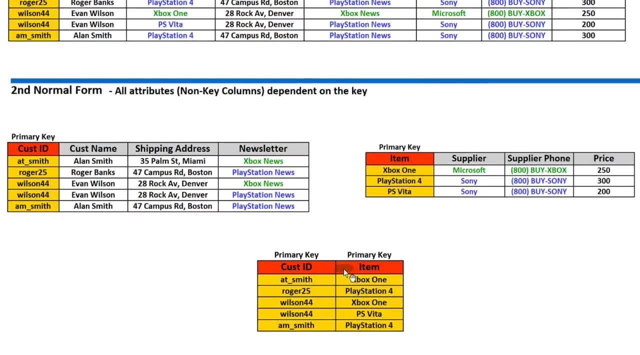 what so? for that, there needs to be a table called the junction table, which is this and basically these in this table. these are both of these are a key. call the compound key because it's made up of two columns. now these entries from 80s 못. box 1 is over. 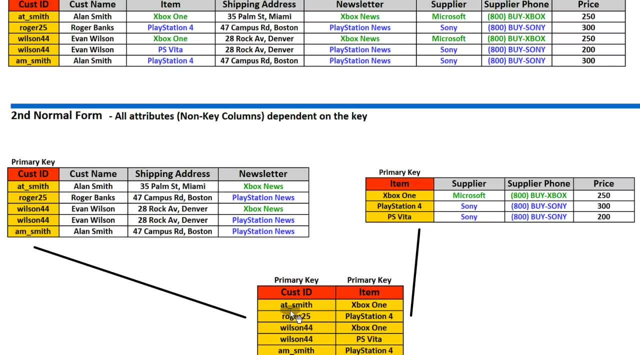 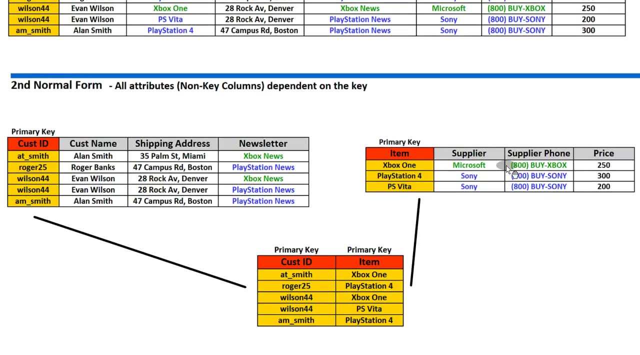 here. so this guy, but this project, 25 by the PlayStation 4, Wilson 44 Xbox one- the video, and am Smith by the PlayStation 4 for. so the transactions are here and now. this and this are lookup table. so, basically, am smith bought an Xbox one, who's a? I'm sorry, 80 Smith, who is that? 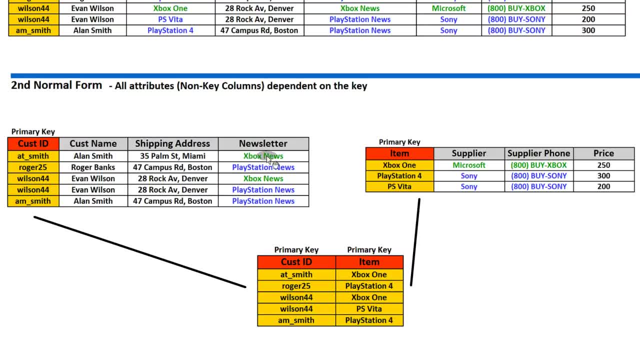 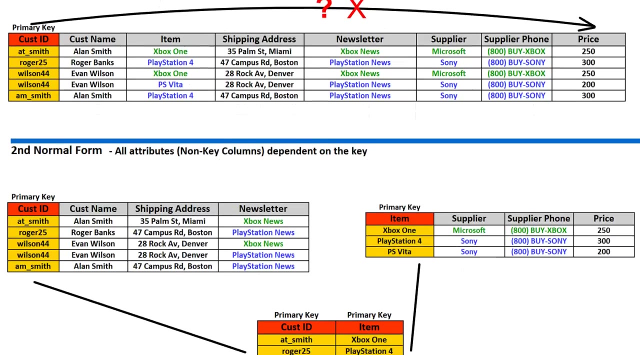 guy. well, his name is this, he lives here and he subscribed to this. what's Xbox one? Xbox one is supplied by Microsoft. this is how you buy more of it if you run out, and this is the price. so this is nine. second normal form, because every, every attribute depends on the key. we separate them out. great. third normal. 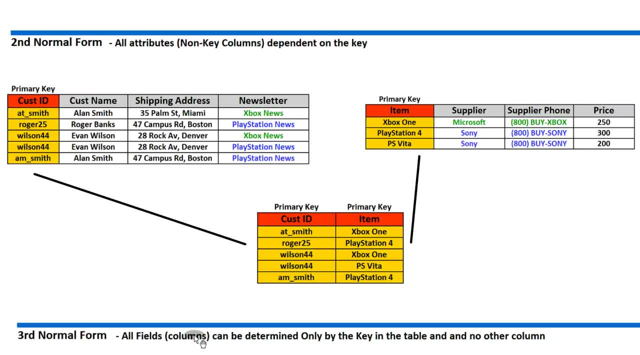 from all fields. meaning columns can be determined only by the key in the table, in no other column. okay, so what can we do? problem here? Well, the problem is that Microsoft and the Buy Xbox phone number always goes together. The Sony and the Buy Sony phone number always goes together. It even says in here: this phone number is never going to go with Microsoft and this phone number is never going to go with Sony. 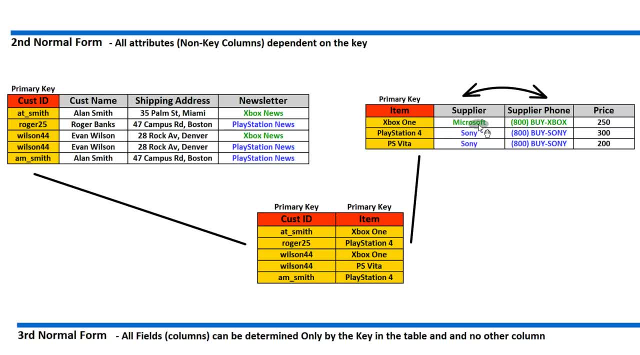 Okay. so in the item table, if the only thing we would know is Microsoft, we already know that this is the phone number. or if we know Sony, well, we know it's going to be just the phone number. So obviously we need to separate it out, also because these phone numbers keep repeating. If I would add more items here, like a camera for PlayStation, a camera for Xbox controller, blah, blah, blah. 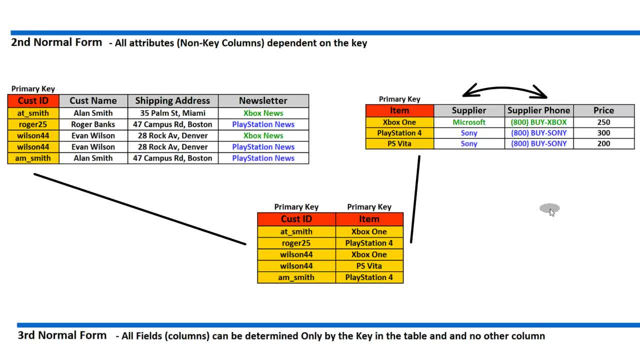 You would notice that Microsoft Sony, Microsoft Sony and their phone numbers keep repeating. So if I would change, if I would have to change the phone number, I would have to change it in a lot of different places and that's not normalized properly. 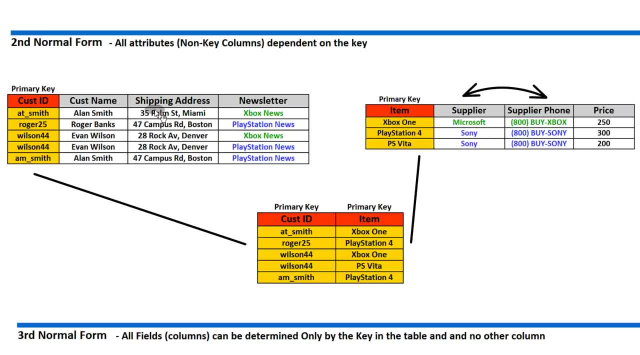 How about here? Can I figure out? let's say, the address from the customer name. Well, Alan Smith is one customer name. There's an address from Miami. Let's see There's another address from Boston. so I guess there is no one-to-one relationship. How about backwards? Let's see, Campus Road goes with Roger Banks. So I guess there isn't a one-to-one relationship between the name and the shipping address. 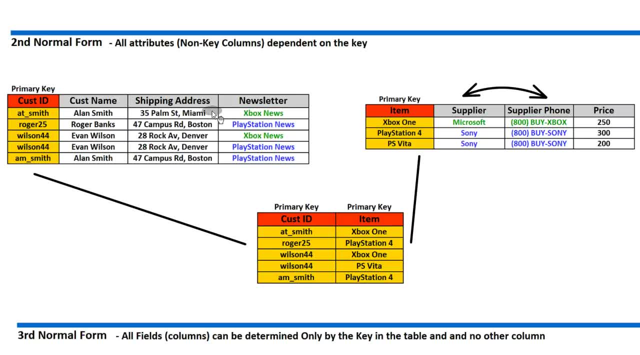 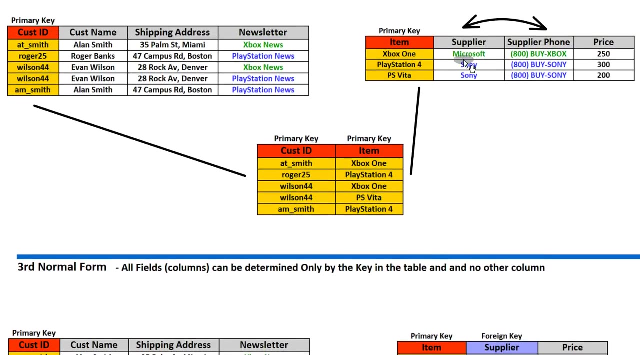 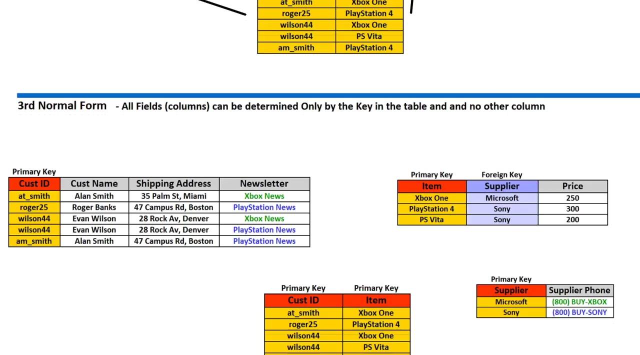 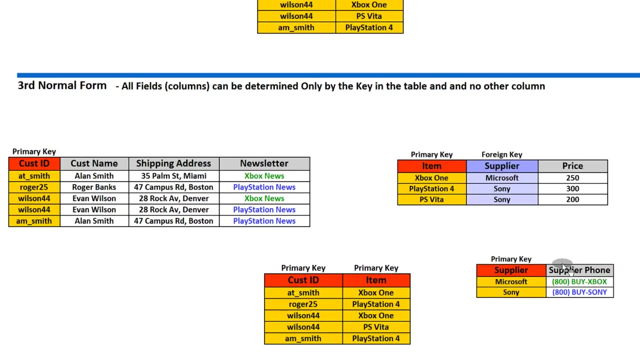 Newsletter. well, that's definitely not going to happen, because a person can sign up to multiple newsletters and multiple people can sign up to the same newsletter. So there's not going to be same relationship as here. We can't just separate it out just yet. So what I did is basically separate this out. This, for now, is going to remain unchanged, but this is separated out. So I would remove the phone number column in here. So now the item is: 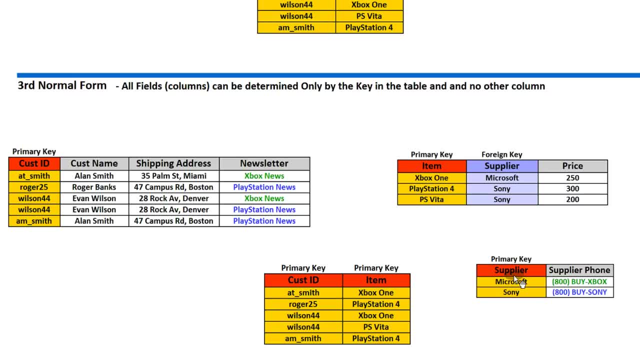 supplied by Microsoft and it's $250, but the phone number is listed here. Now, if I need to change the phone number for either one of these, I can do it in one place and there's no redundancy. Obviously, the supplier is now its own primary key in its own table and is a foreign key in the item table. The foreign key is the one that was located in the item table, So I can delete this and I'm nice and simple. That's all I can do. 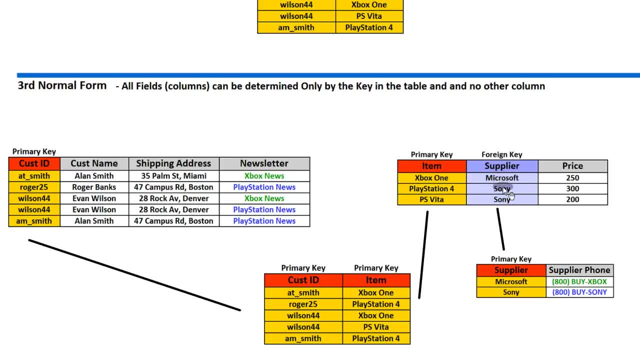 key simply means that in here you can only enter values that appear here. if it's not in here and not in this table, you cannot put it in here. let's say, if you want to put in supplier revlon or l'oreal or something like that, those are not. those supply cosmetic products or whatnot. so they, if you. 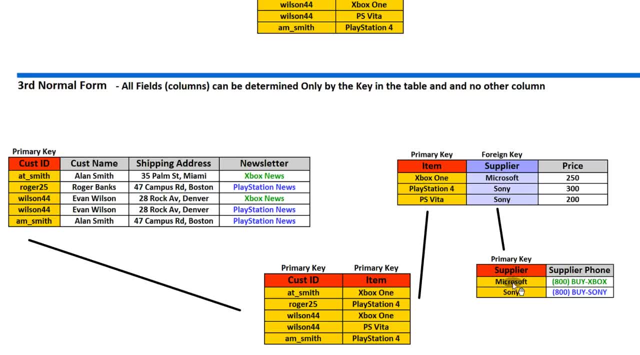 don't sell those. you can't just enter in here. it has to be in the supplier table first before you can put it in here. that's what the foreign key means. okay, so now all columns can be determined only by the key in the table and no other column. well, this side is done for sure. there's no, no. 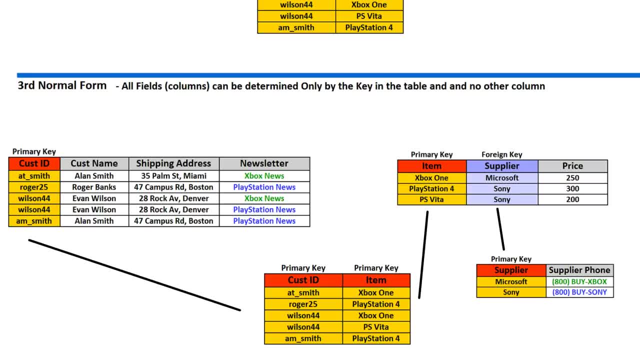 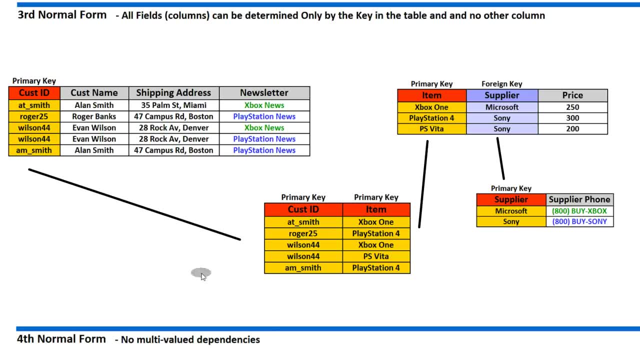 further way to normalize it. there's only this side left. so fourth normal form: no multi-value dependencies. well, what does that mean? what's a multi-value dependency? it's basically this: this field depends on the customer id, this address depends on the customer id and the subscription depends on the customer id. 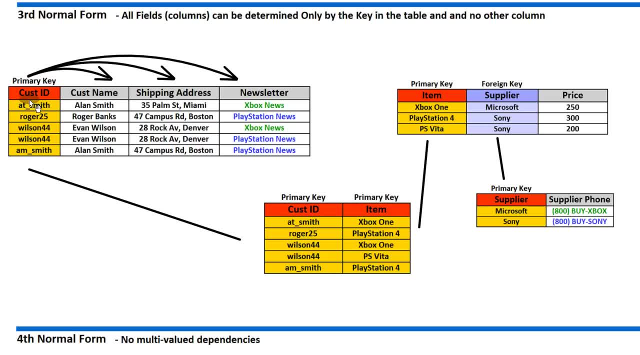 so these are all dependencies of the key. however, there's still a problem. as you can see, evan wilson is in here twice with the same address because he subscribed to two different newsletters. so if he would change his address, i would have to change it two places. 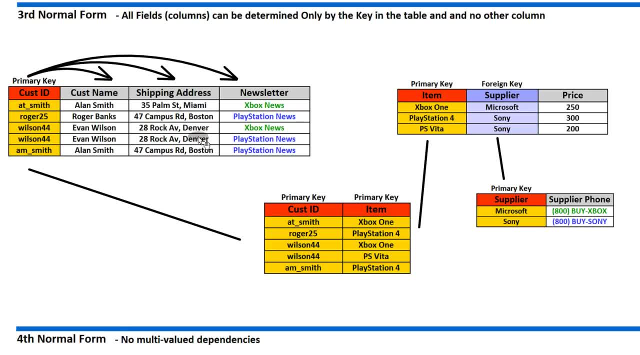 or what if he would unsubscribe to this thing then then what? do i just put a null here or try to declude my database? uh, because now i have uh two entries, or what? if you unsubscribe for both of them, then i'm gonna have two nulls and two of the same. 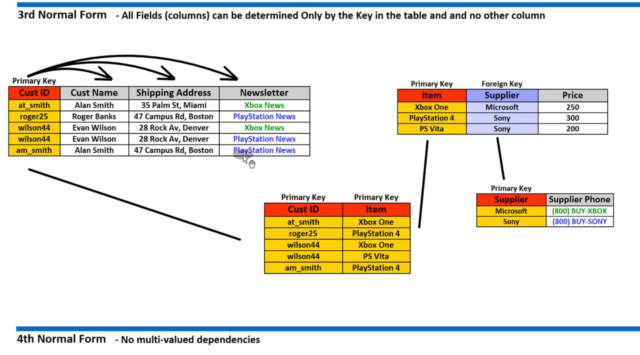 values or same thing. if, if this person signs up for a new the xbox newsletter, i repeat his user id and the customer name and shipping ad is just just basically like you either leave it as null or just randomly repeated, because what are? what are you going to put there? so the multi-value dependency is a situation where one column can have different values, a different amount of values than, let's say, the other column. for example, in this database i didn't allow multiple shipping addresses per customer. every customer has one shipping address, but they have multiple newsletters. but in real life, let's say, if you have an amazon account you can have multiple, let's say, credit card numbers on file and the checkout. 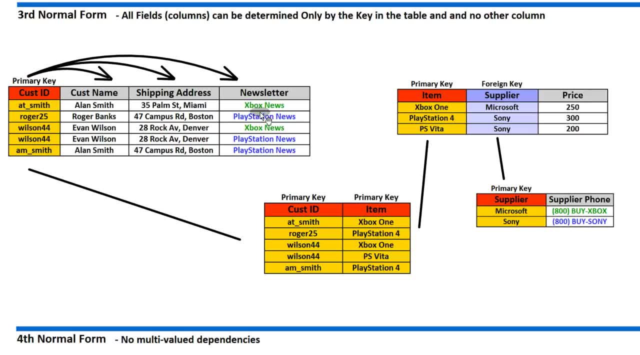 at checkout you choose which one you want to use, and you could have multiple shipping addresses, one home, one for work. so for one person you could have, let's say, two shipping addresses and four credit cards. well, how do you make a proper table out of that? the amount of rows in this column is not the same as in this column, let's say, for. 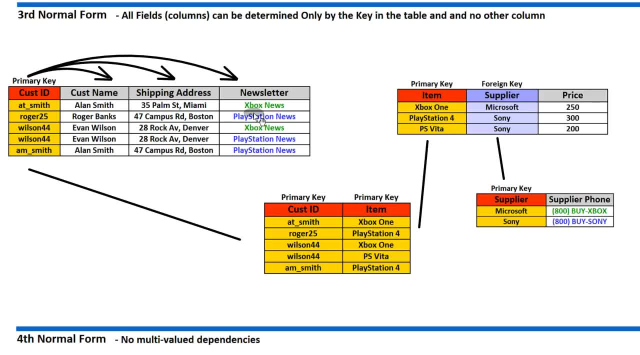 example, I would have one shipping address and two credit cards and then I would add another shipping address. what would I put in the credit card field? just randomly select one of them. you see how that's. that's a situation where you have these fields depend all on the key and which is called the multivariate. 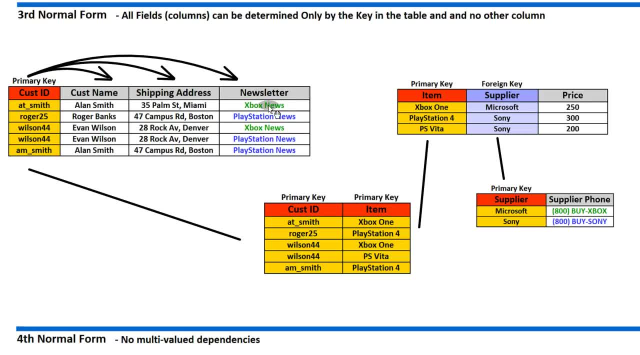 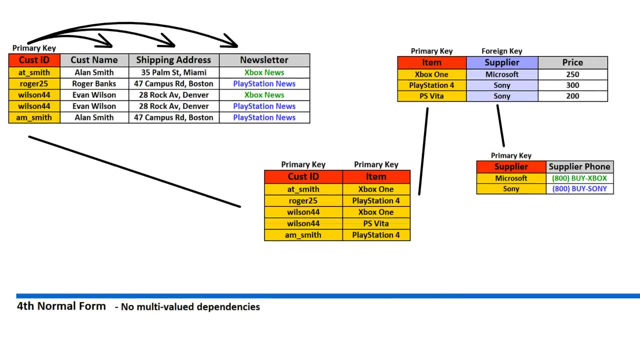 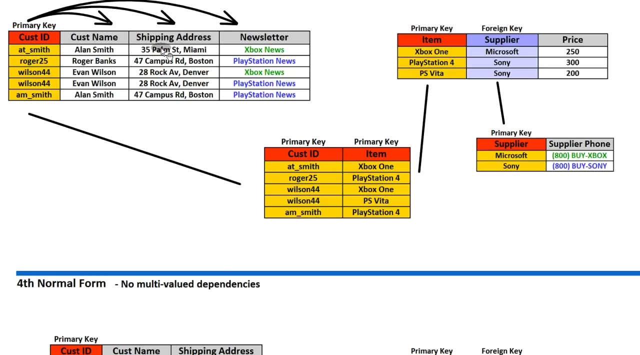 dependency, but there's different amount of values that can be put into each row. I mean- I'm sorry- in each column. so obviously at this point this needs to be separated out and what I separated out is the customer ID. customer name and the shipping address is gonna be one table and the newsletter and the customer ID will be. 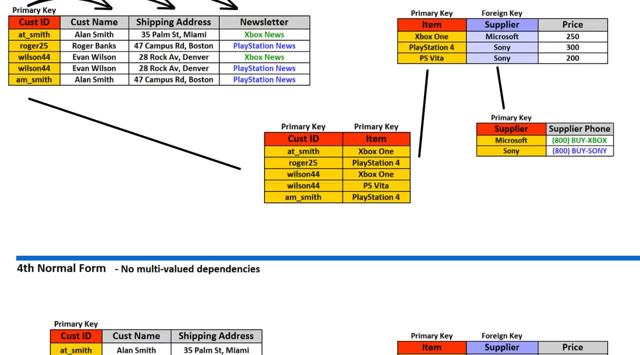 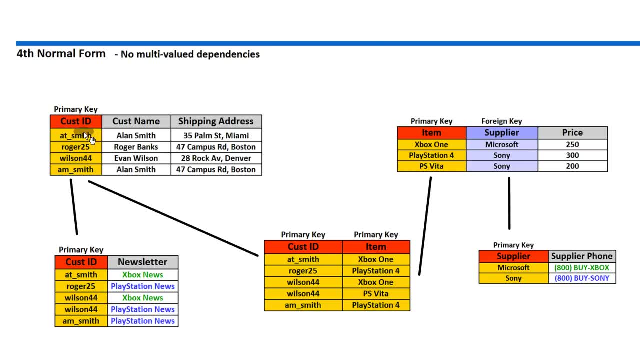 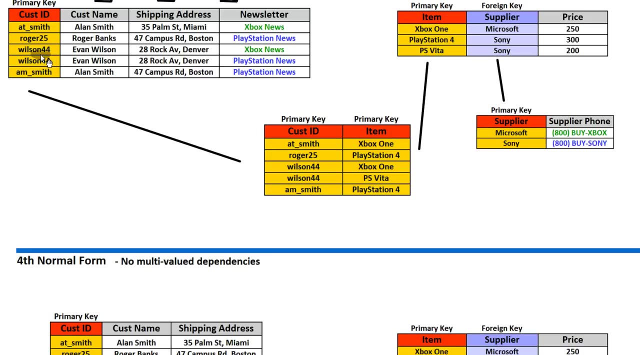 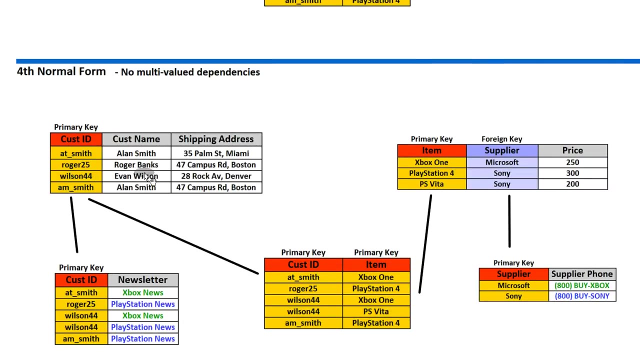 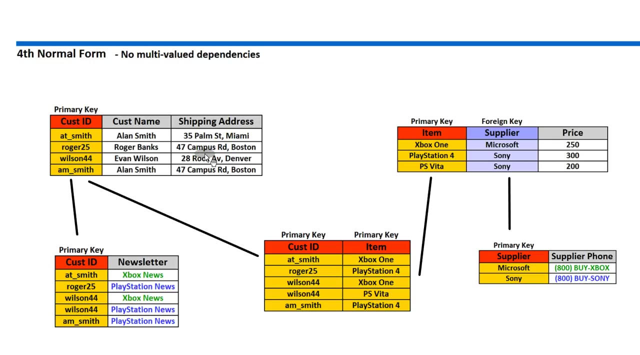 another table. this: these remain the same. so as you can see, now every customer only appears once. Wilson44.com was eliminated twice because we don't need that, so now if I need to change his address, he's only in here once. I don't have to change it twice. and these are: 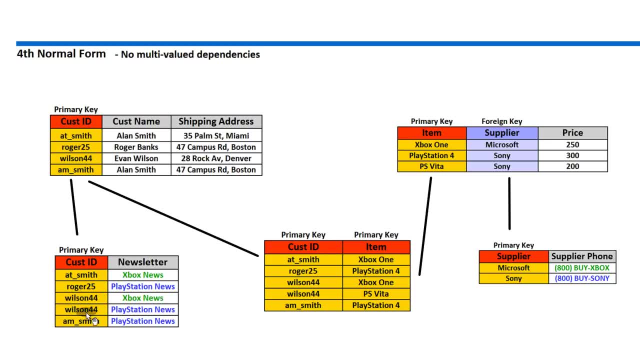 his subscription. he's in here twice. so if the query that returns the who- what kind of newsletters need to go out? will return him properly, because he'll be in here twice. if this person signs up to another one, who'll be in here twice and the query will return it accordingly. or, let's see, 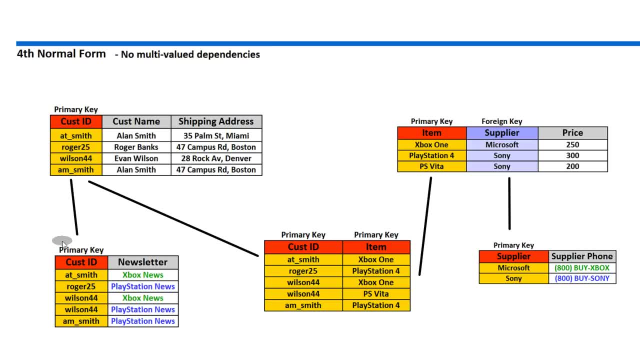 Roger, on subscribes, he'll be removed and the query that returns the newsletters will not return his name, but his address will be still intact here, no problem. these other relationships between the tables and. and also gave the tables names because now I know what they are, so this means this one too many, this. 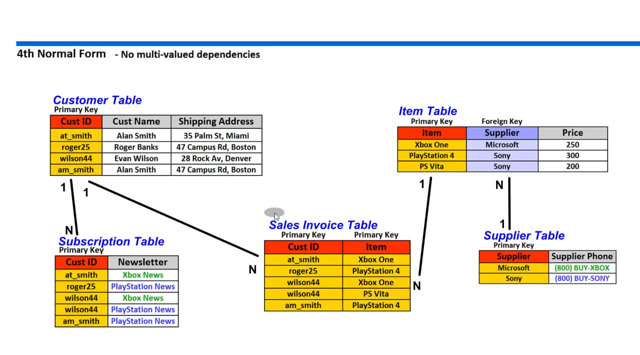 means the customer appears in this table one time, but in the sales invoice table he will appear multiple times. an item will appear one time in the items table but will be sold multiple times. supplier will appear one time but can supply multiple items and the customer will appear. 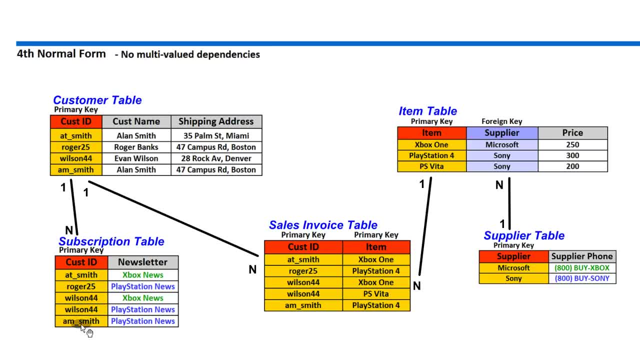 one time here. but he, the person, can have multiple subscriptions or not at all, none at all. so now this table is fully normalized and thanks for watching.